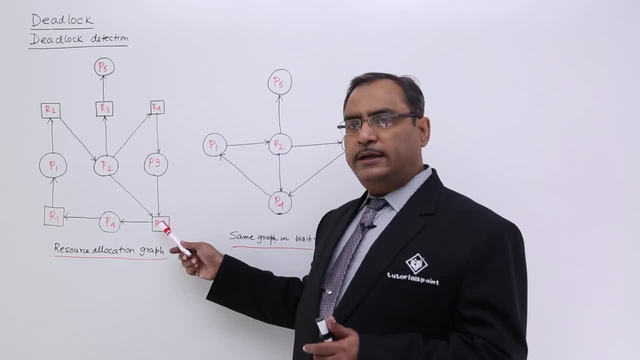 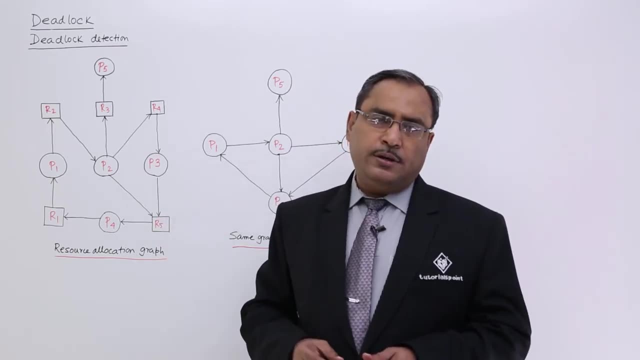 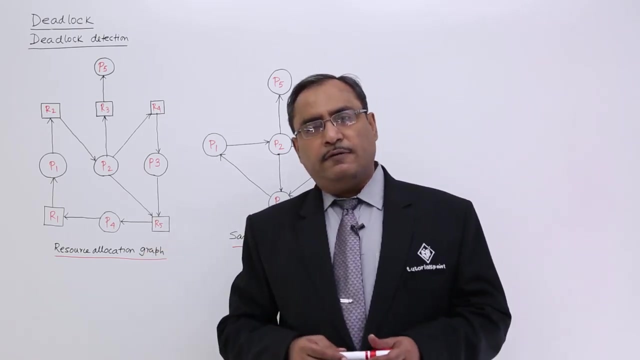 request edge And some edges will be directed from resource to the process, will be known as the allocation edge. So request edge, allocation edge process and the resource are the four components. Now we know that in case of resource allocation graph, if there is no cycle, cycle means closed. 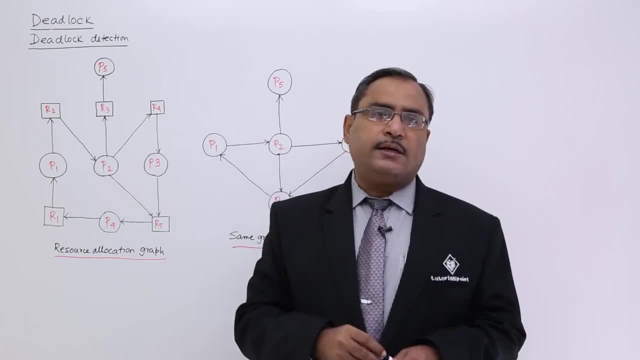 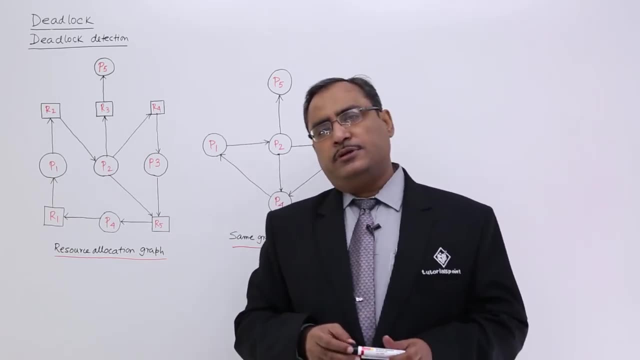 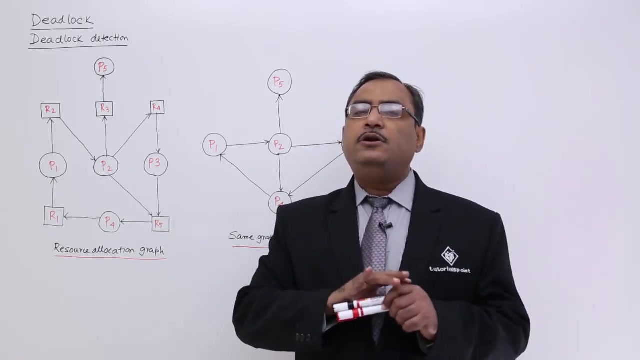 path, because all of these arcs are edges, are directed. So if you go through the directions and if you get a closed path, then you can say that this particular resource allocation graph is having one cycle. So if a resource allocation graph is cycle free, that means deadlock will not occur. 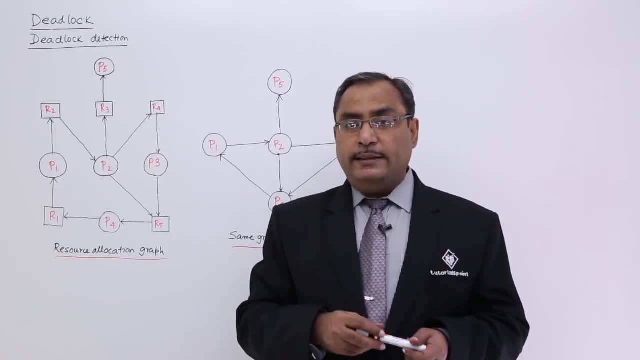 But if the resource allocation graph is having one cycle, all events of same process will occur. So that is all it can do. And for all block位 there will be a request edge чуть having a cycle. then deadlock may or may not occur. so each and everything we discuss in 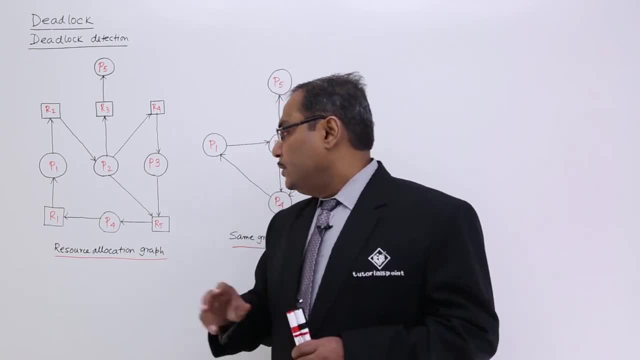 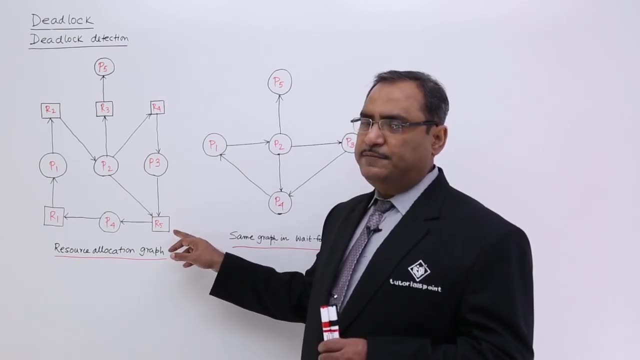 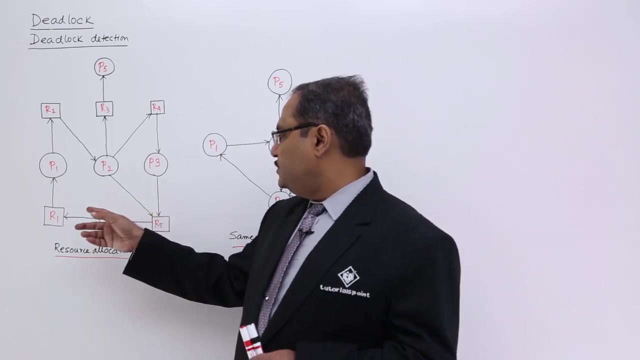 our previous videos. please watch them. so now i cannot ensure myself that deadlock is going to take place. if cycle exists in resource allocation graph, let me check whether here we are having any cycle or not. let me check once. so we are. if we move in this way, we are. 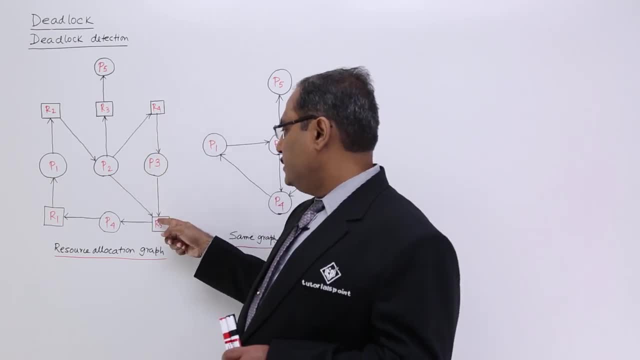 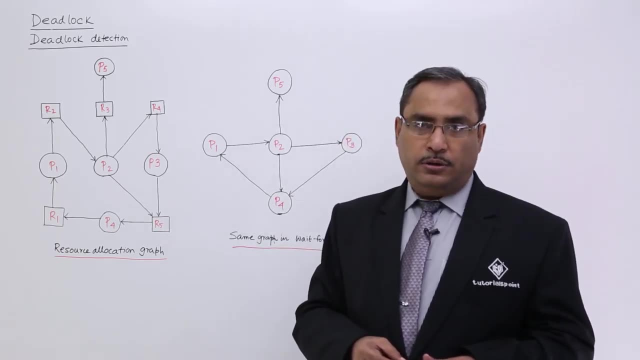 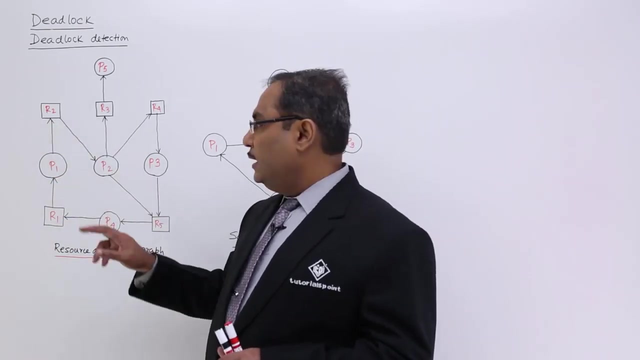 getting this? we are getting this. yes, i am getting this. yes, yes, that is a closed path, so cycle is existing, but i cannot ensure whether deadlock is occurring or not. so let me check why the cycle is there. you see, p 1 has got r 1 waiting for r 2. p 2 has got r 2 waiting. 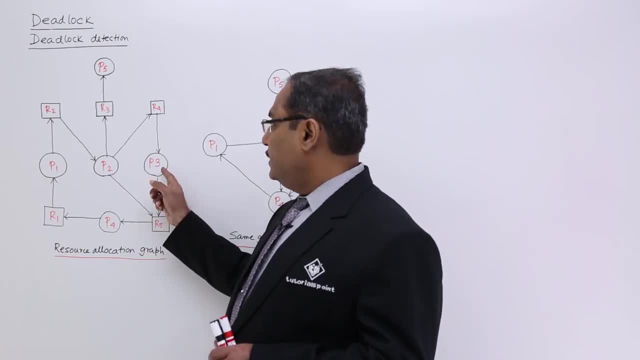 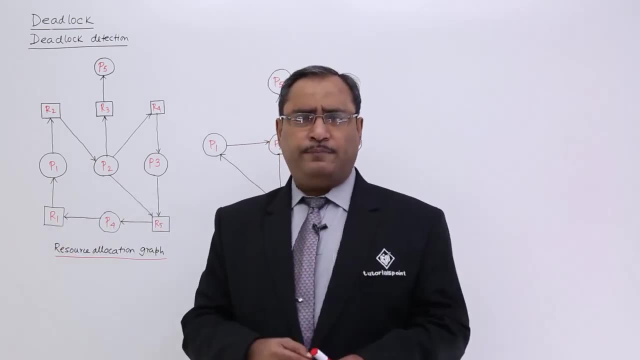 for r 3, r 4 and r 5. p 3 has got r 4, but waiting for r 5. p 4 has got r 5, but waiting for r 1. so everyone is waiting. everyone is either for the one resource or for more than one. 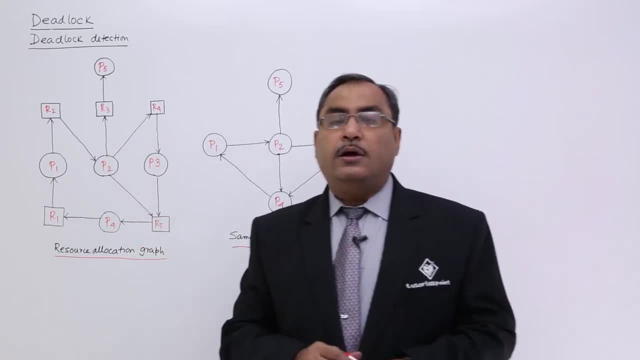 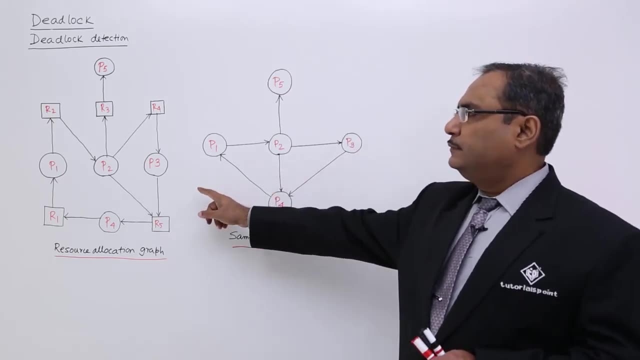 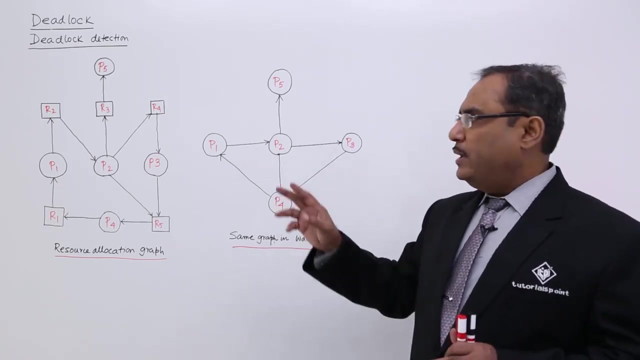 resources. they are waiting, so cycle is there. now let me convert this resource allocation graph with the respective wait for graph. this is the same graph has been represented in the wait for graph. remember this one that in case of wait for graph, we do not have the resources, we have only this directed edges and the processes enclosed within circles. 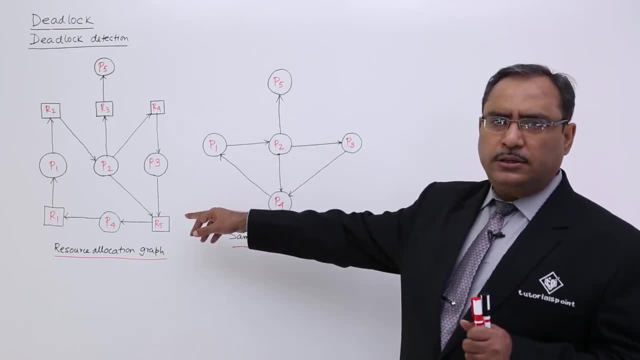 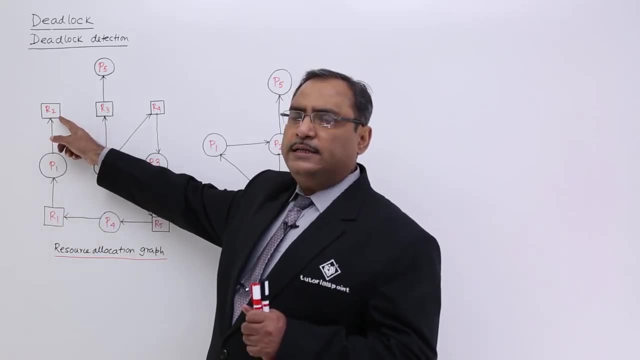 now why this graph has got formed from that particular resource allocation graph. let me tell you. you see, p 1 has got r 1 waiting for r 2. why r 2 it is not getting? because r 2 has got already been allocated to p 2, so actually p 1 is waiting for the completion. 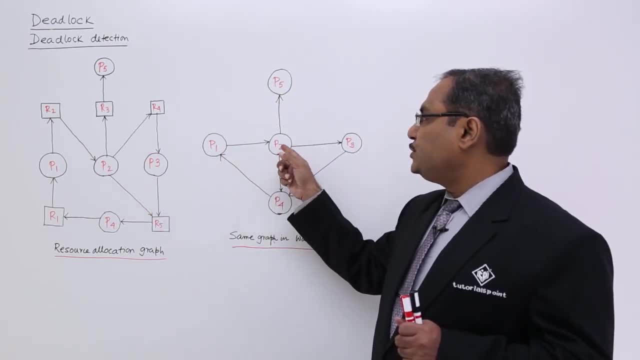 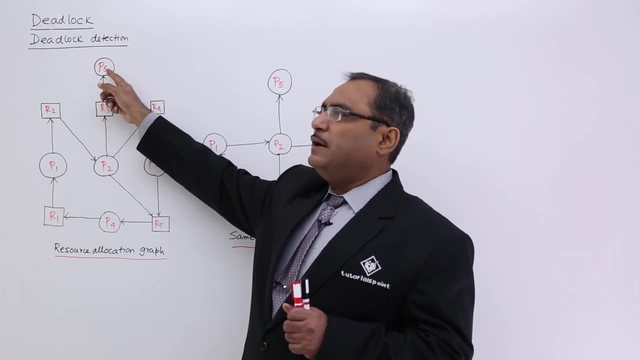 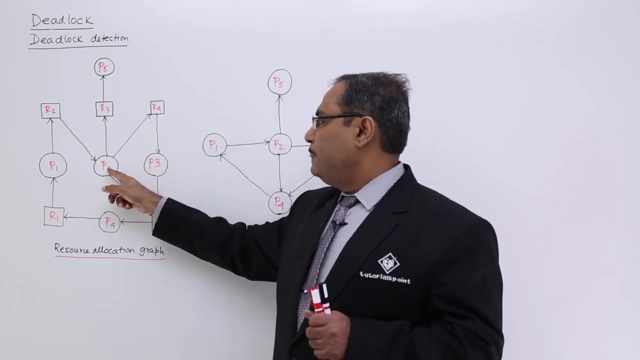 of p 2. so p 1 is waiting for the completion of p 2. good next, p 5 is waiting for none, because p 5 has got the instance r 3.. And it is not waiting for none, so p 5 is waiting for none, good. next go for p 3. p 3 has got r. 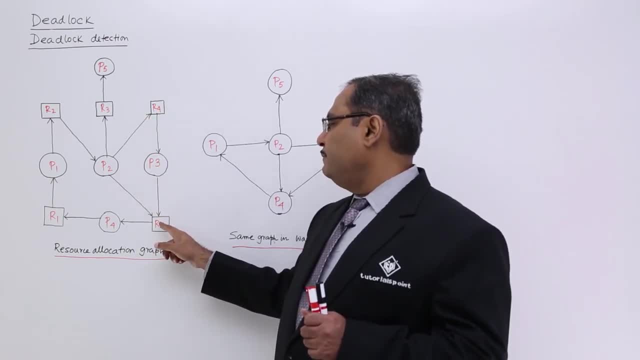 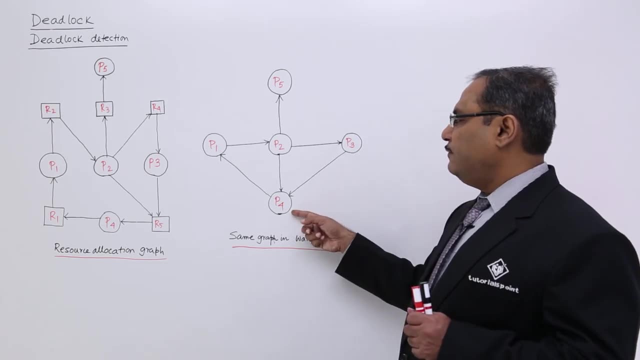 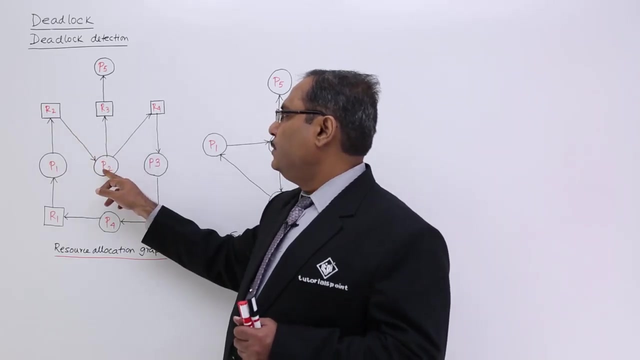 4, but waiting for r 5. and r 5 has got allocated to p 4. so p 3 is waiting for p 4s completion. so p 3 is waiting for p 4s completion. Let me go for the p 2. at last now see, p 2 has got r 2, but waiting for r 3. r 3 got allocated. 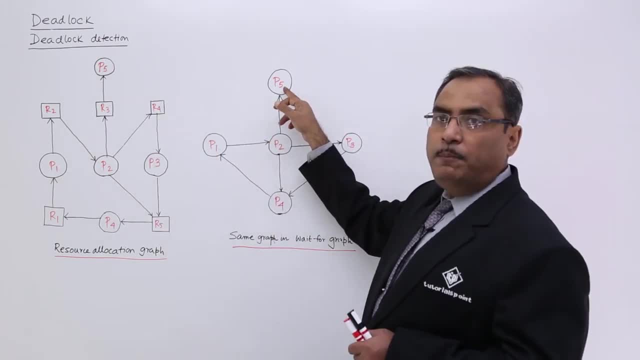 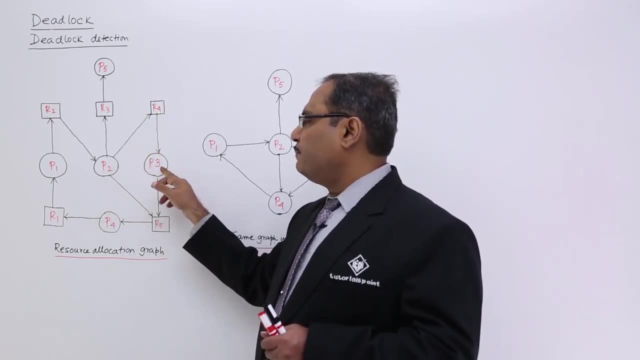 to p 5.. So p 2 is p 2 is waiting for the completion of p 5. p 2 is waiting for r 4. r 4 got allocated to p 3, so p 2 is waiting for p 3s completion. so p 2 is waiting for p 3s completion. p 2: 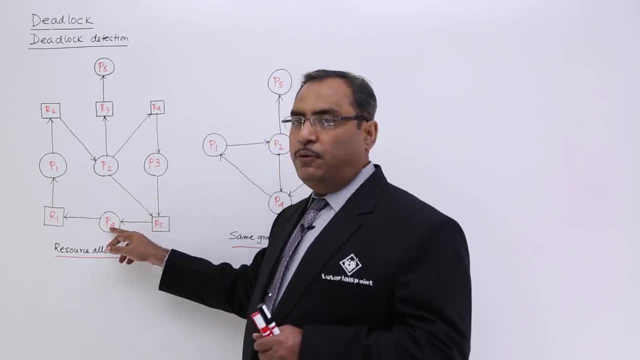 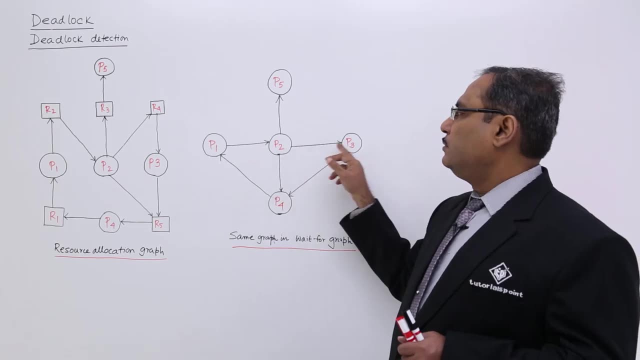 is also waiting for r 5 and r 5 got allocated to p 4. so p 2 is waiting for p 4s completion. so p 2 is waiting for p 4s completion. so 3 outward edges are coming out from p 2.. 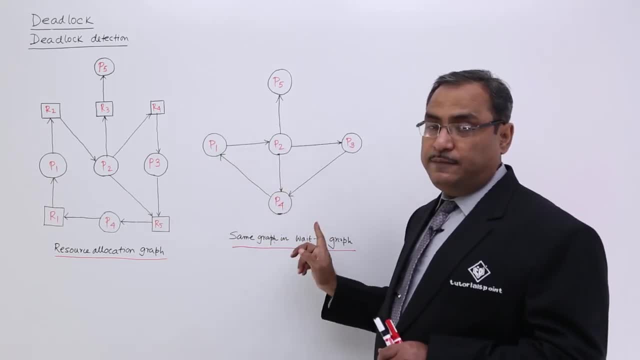 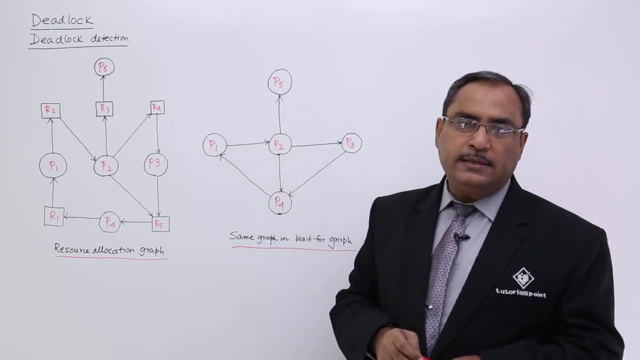 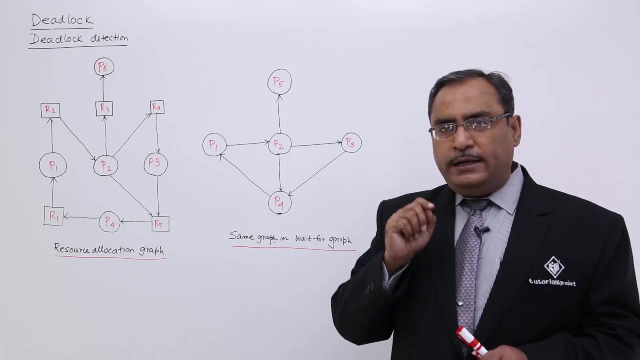 So this is the respective wait for graph. this graph is having the name wait for graph. So who is waiting for whom? So that graph is actually depicting the same. In the wait for graph, if you find a circle with a, not if you find a circle or cycle. 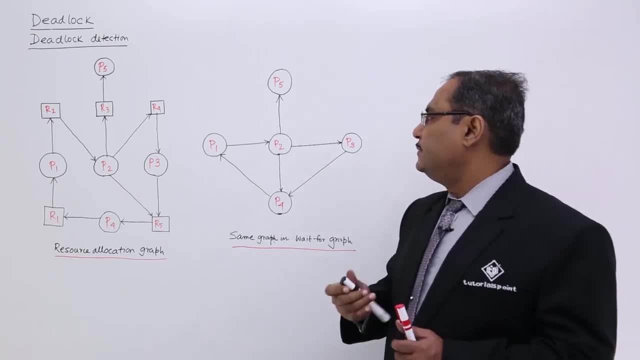 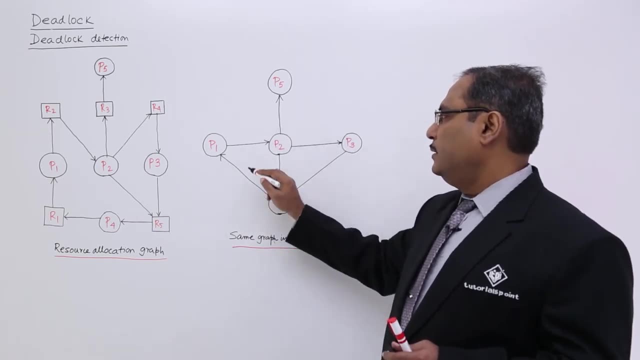 with a not, then deadlock is bound to take place. Just see, here we are having one cycle. this is the cycle is there and there is a not type of thing. So there is a cycle and there is a not type of thing. that means deadlock is bound to.